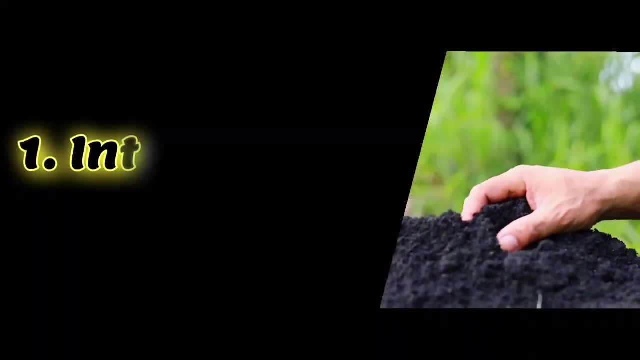 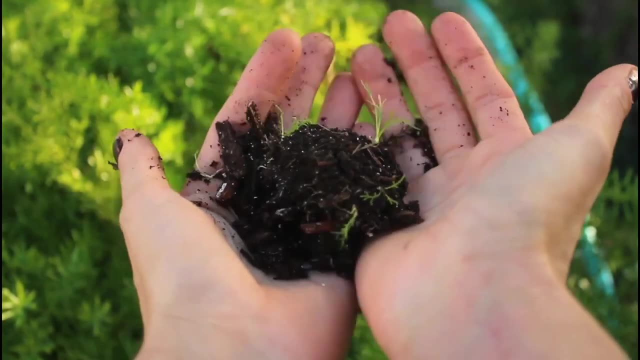 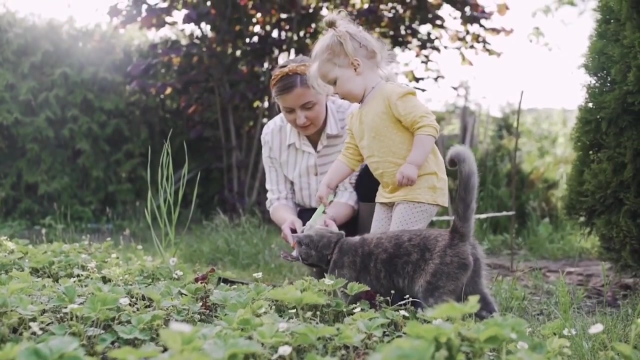 the journey from rocks to rich, fertile soil. 1. Introduction to Soil. Soil is a remarkable blend of minerals, organic matter, air, water and countless microorganisms. It's the foundation of life on land, supporting plants, animals and even us. 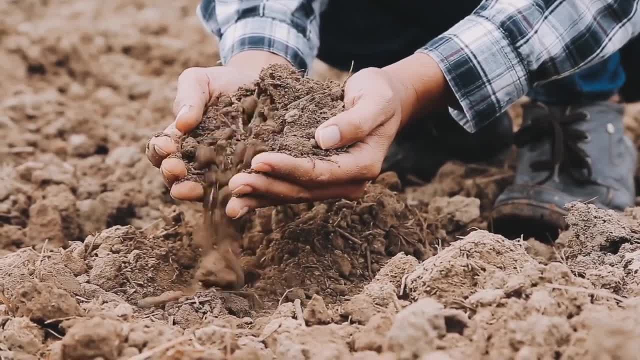 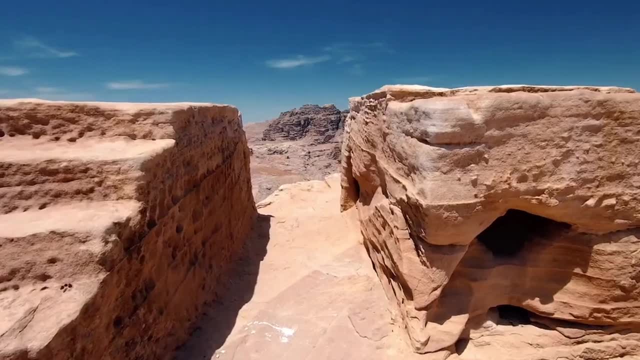 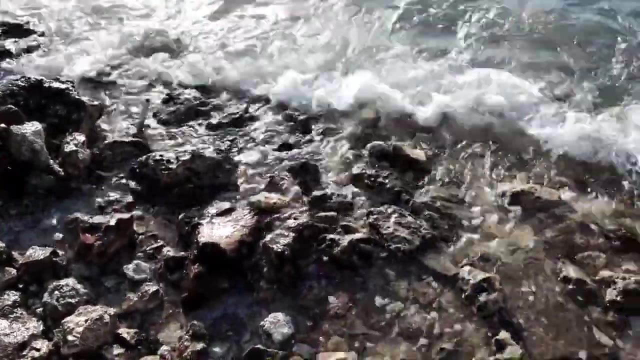 But have you ever wondered how this magical mix comes into existence? Well, it all starts with the earth's crust. 2. Weathering Rocks. Our journey begins with rocks, the building blocks of our planet. Over millions of years, rocks are exposed to the elements such as wind, rain. 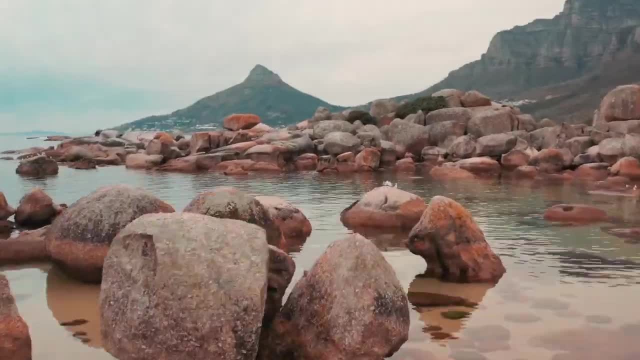 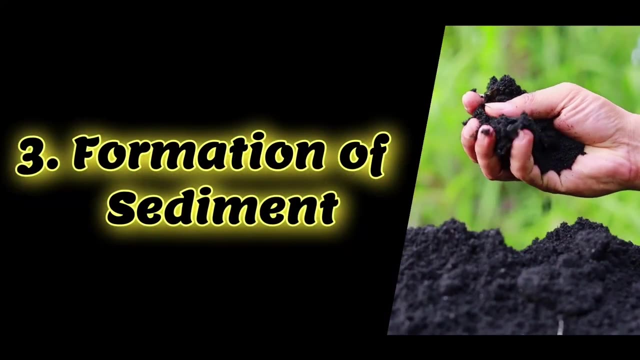 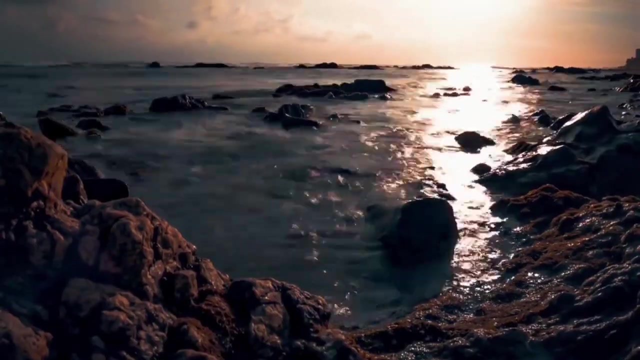 and temperature fluctuations. This process, called weathering, breaks rocks down into smaller particles. 3. Formation of Sediment As rocks erode. the resulting tiny mineral fragments and particles are transported by water and wind. These particles settle in various locations. 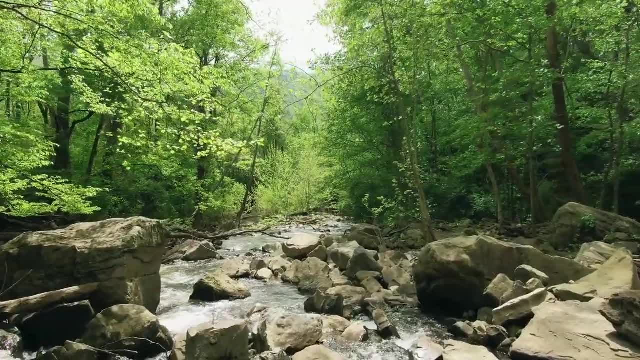 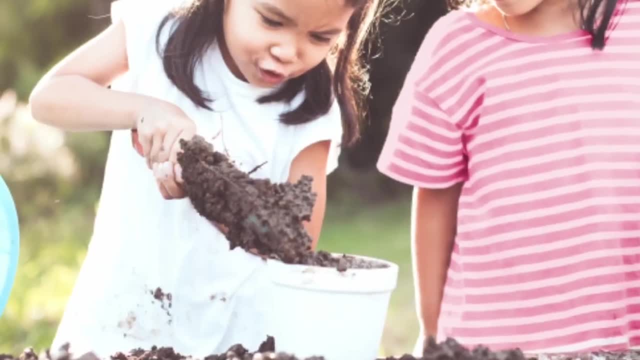 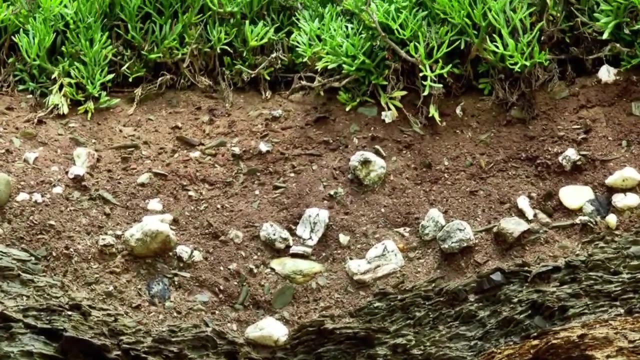 creating sedimentary layers. Over time, these layers build up and become sedimentary rocks. 4. Decomposition and Organic Matter- Now here's where things get interesting. transform sediment into soil. we need the magic touch of organic matter: Leaves, plants and other. 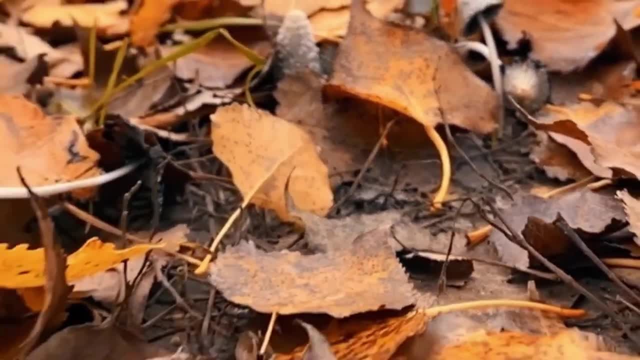 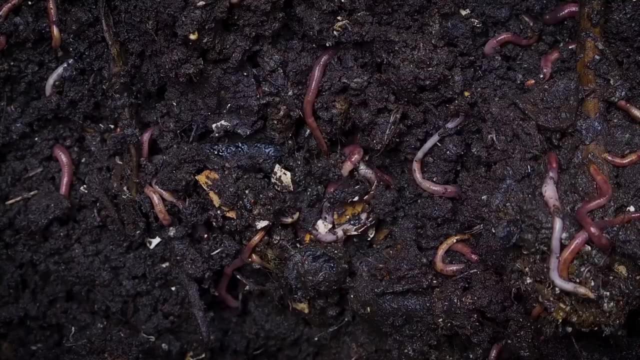 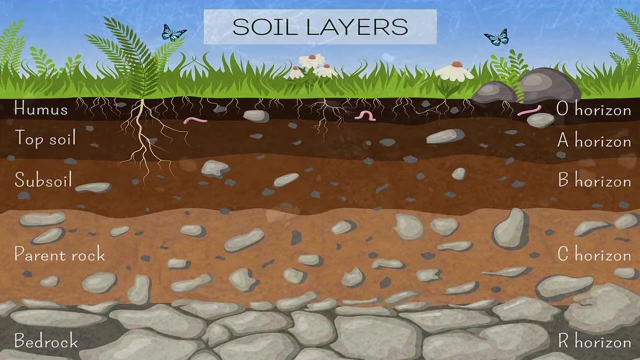 organic materials fall to the ground and start to decompose. This process enriches the sediment with nutrients and creates the dark, nutrient-rich layer we know as topsoil. 5. Soil Horizons. Soil isn't just a uniform substance. It's composed of different layers or horizons. 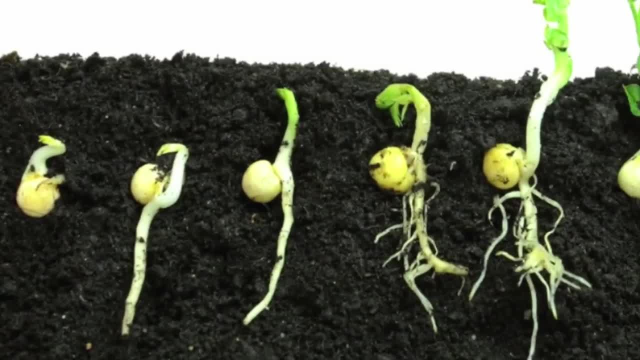 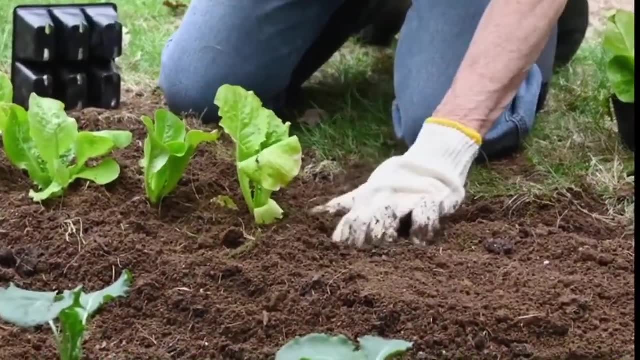 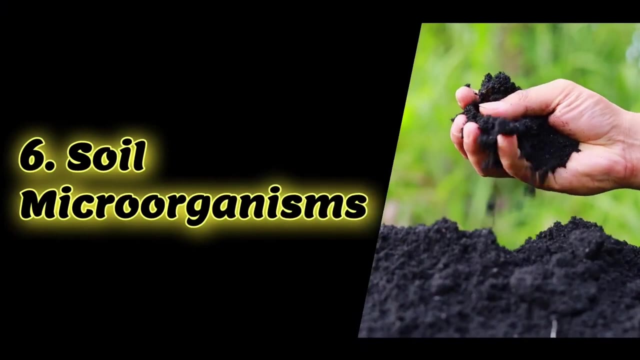 each with unique characteristics. The topsoil is where most plant roots thrive, while the subsoil contains minerals leached from above. Understanding these layers is crucial for successful agriculture and gardening. 6. Soil Microorganisms. One of the most remarkable aspects of soil is the thriving world of microorganisms that call it. 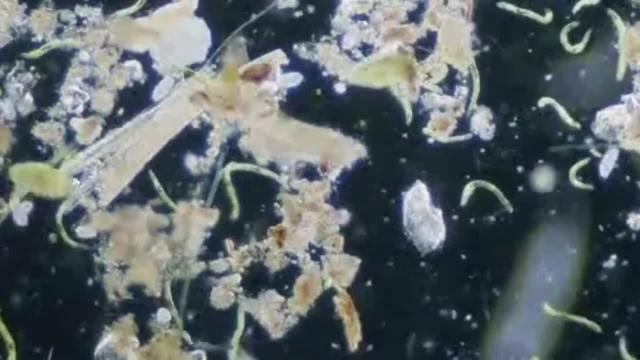 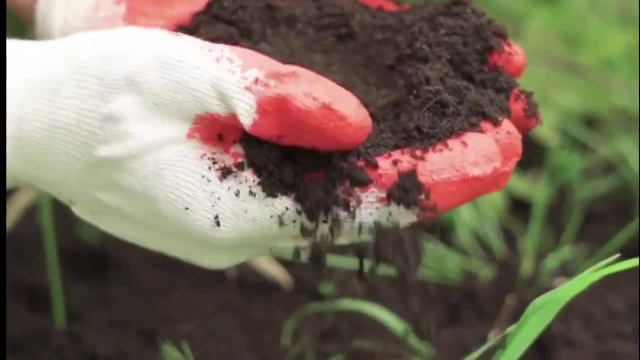 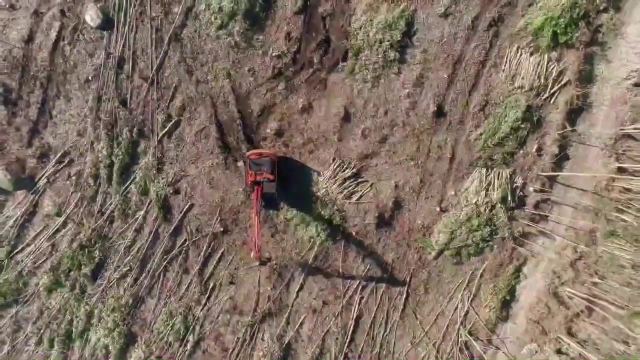 home. Bacteria, fungi and countless other tiny creatures break down organic matter releasing and then they are destroyed. Soil is the most remarkable aspect of soil. 7. Human Impact. Unfortunately, human activities like deforestation and unsustainable agriculture practices can